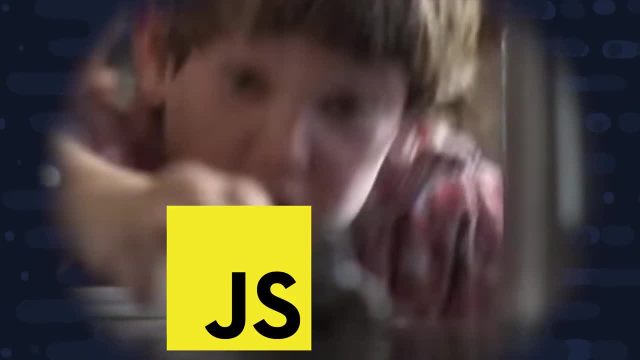 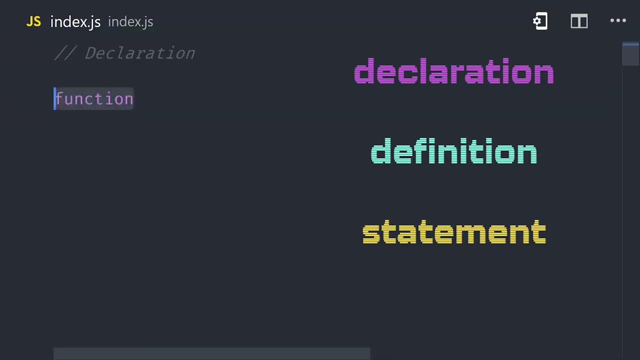 looking at its anatomy. What we're looking at here is a function declaration, also called a function definition or statement. It starts with a function keyword. then you need to choose a name for it, And you should choose something that's readable to other human. 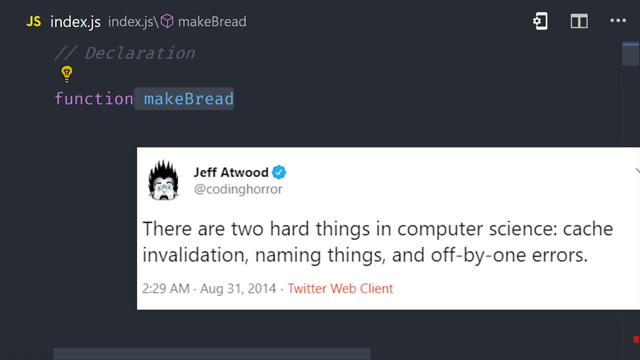 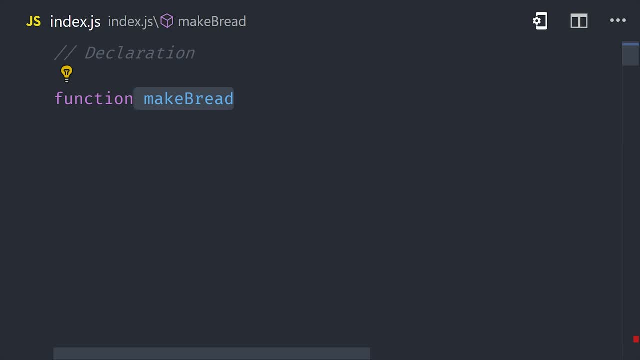 beings. because there's a good saying: there's only two hard things in computer science: cache and validation. In other words, choosing the right name for your function is almost as hard as making a joke about programming. But once you decide on a name, the next step is to add parentheses. 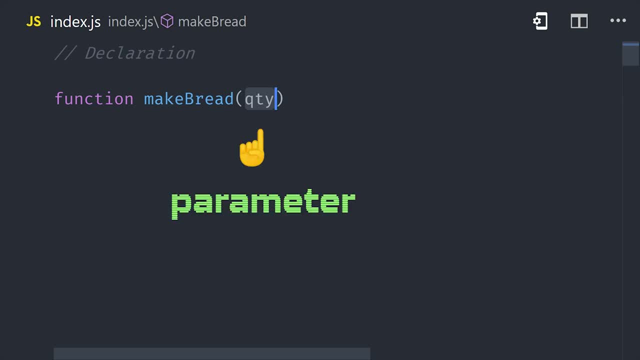 and then add any parameters or inputs to the function. You can think of a parameter as a variable that this function will have access to when it's called, And then from there we have curly braces and everything inside is the function body, And that's where you define. 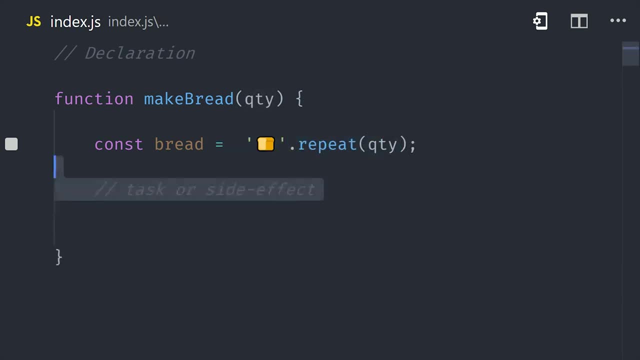 all your logic. The function body will typically do one of two things. It will either perform a task or return a value, or possibly both. An example of a function performing a task is a console log, and because there's no return statement, it will implicitly return undefined. But a function body might also. 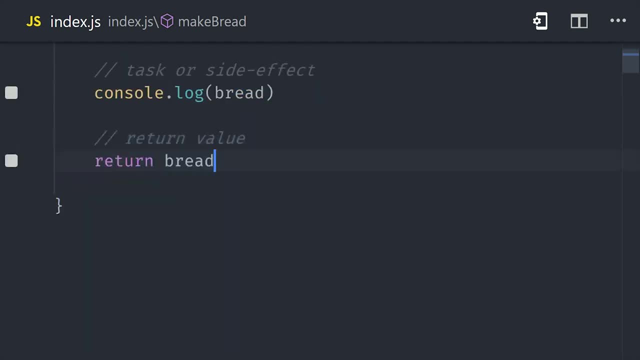 contain a return statement, and that allows us to take the value that was calculated inside the function body and set it as a variable. Now, at this point, we've declared a function which describes what the code will do, but in order to actually execute it, we need to. 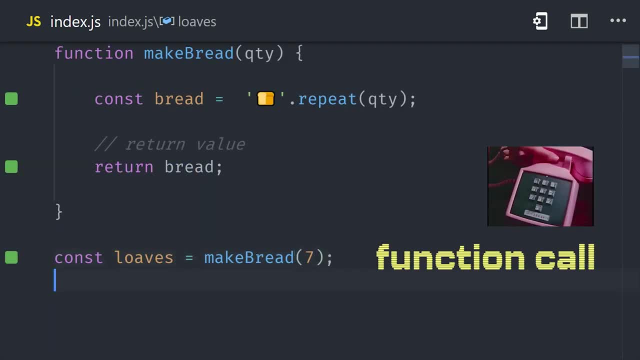 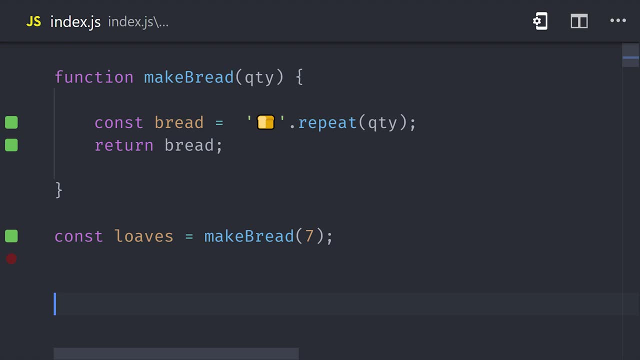 call the function. We do that by referencing the function by its name and then we pass in actual values as arguments to the parameters. So imagine you get asked on an interview: what is the difference between a parameter and an argument? You might say something like: 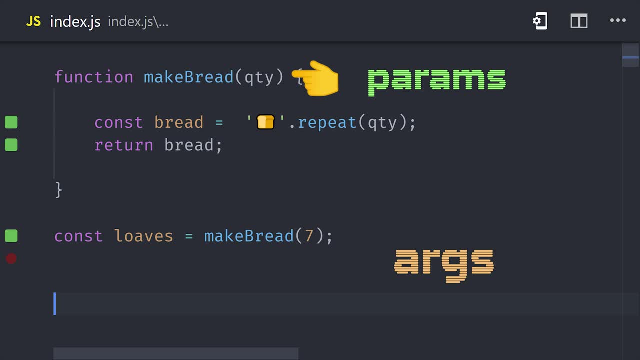 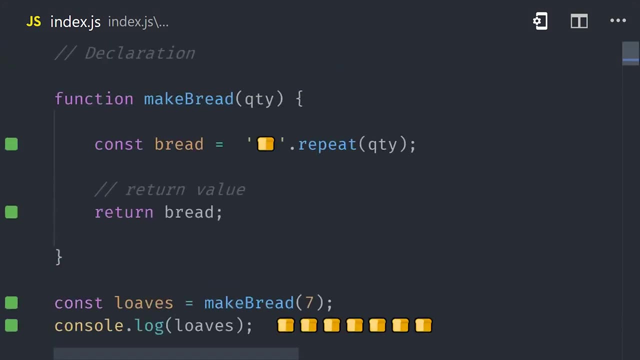 parameters are the variable inputs that you use in the function definition, while arguments are the actual values or expressions used when calling the function. So what we just looked at there was a named function declaration, but there's also a thing called a function expression, which basically means using a function as a value. Let's go. 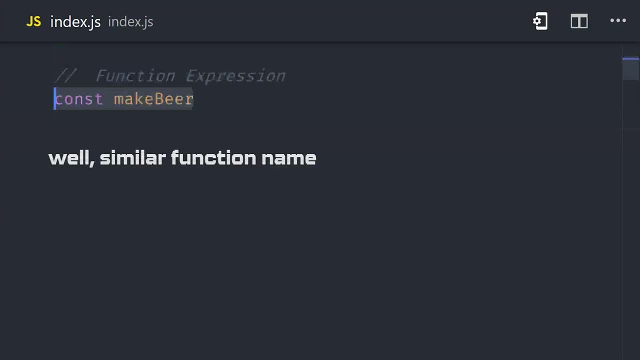 ahead and refactor our declaration to an expression. We'll use the same function name, but instead set it as a variable and then use an anonymous function which is just a function without a name as the value. Now, when calling these functions, they will produce an identical result. and if you watched, 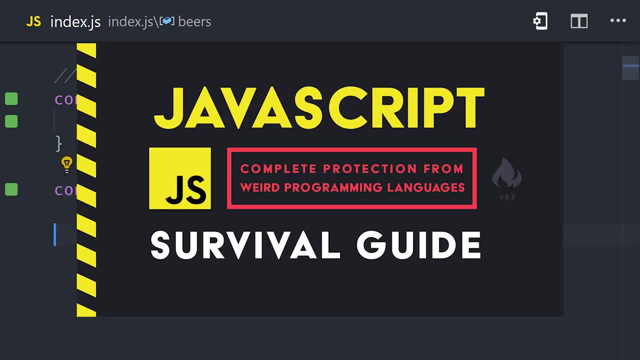 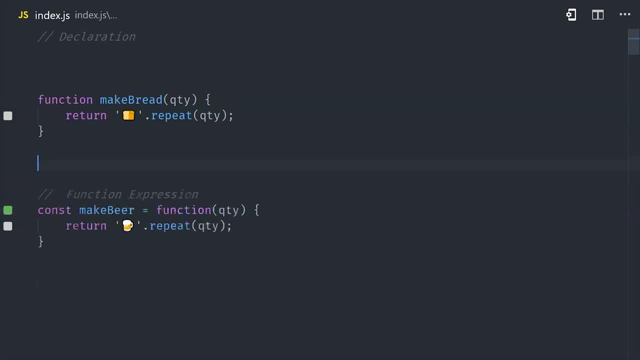 the previous video, you might know that the function declaration is hoisted while the expression is not. The function declaration will always be put at the top of the scope, which means you can make calls to the function even if it's declared somewhere later in the. 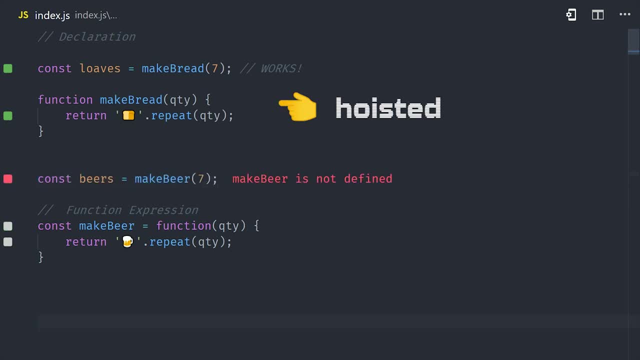 code, But when you have an expression, the function doesn't actually get created until that code is reached in the script, and that means you get an error if you try to call it beforehand. So now that you know the difference between a function declaration and expression. 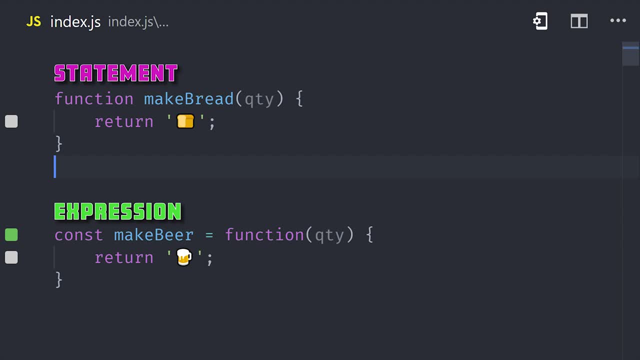 which one should you use? Well, there's actually no universal best-priced function declaration. but there's actually no universal best-priced function declaration. Well, there's actually no universal best-priced practice here. but I think most people today would lean towards function expressions Because 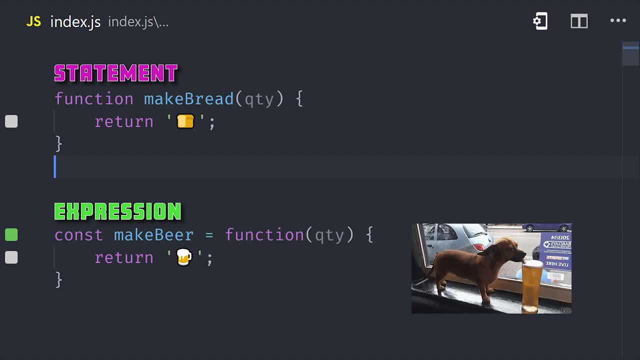 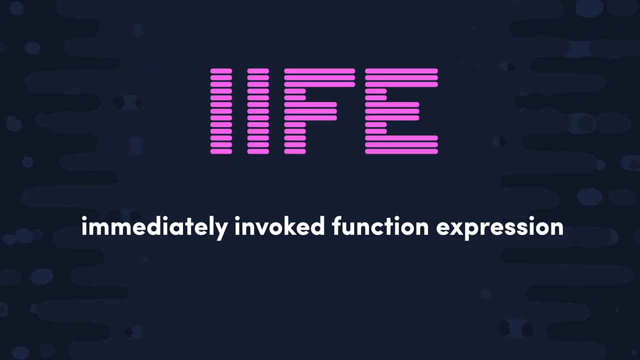 they're not hoisted, it makes it easier to understand where they belong in the context of an application and they're less likely to pollute the global namespace. And, speaking of that, a cool thing you can do is create an immediately invoked function. 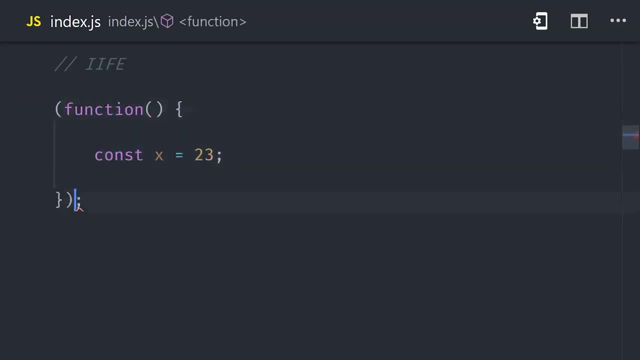 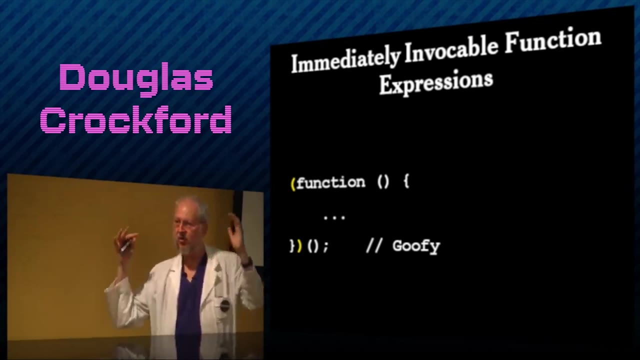 expression By wrapping an anonymous function in parentheses. you can then call it immediately by adding parentheses afterwards. But I think that looks goofy, because what we're talking about is the whole invocation, but we've got these things hanging outside of it, looking sort of like: 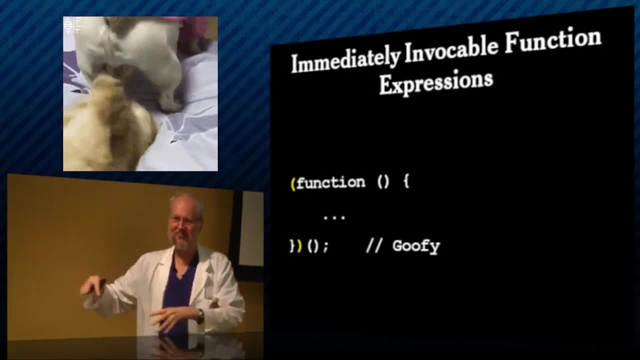 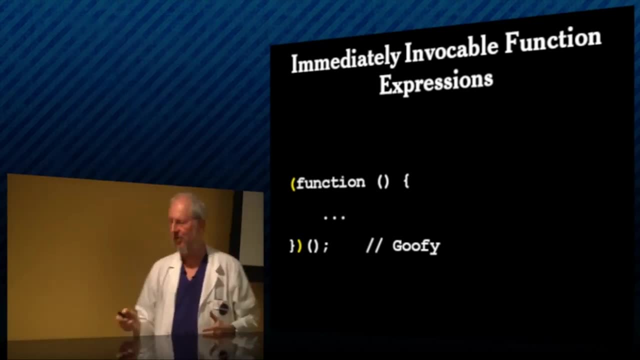 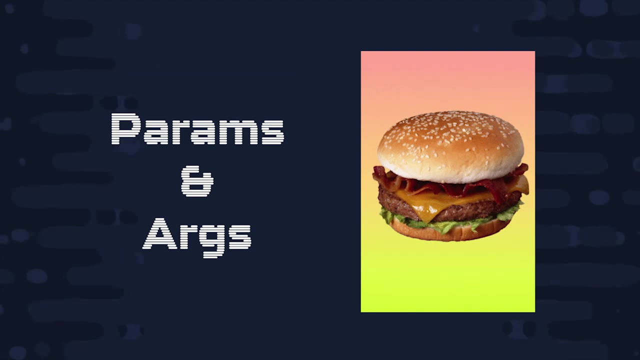 dog balls. you know What's important is the whole invocation, so I would put the parents around it. That's better, I think. So now let's go ahead and switch gears and take a closer look at parameters and arguments. As you can see, here we have three parameters: a main, a side and a drink. And if we want, 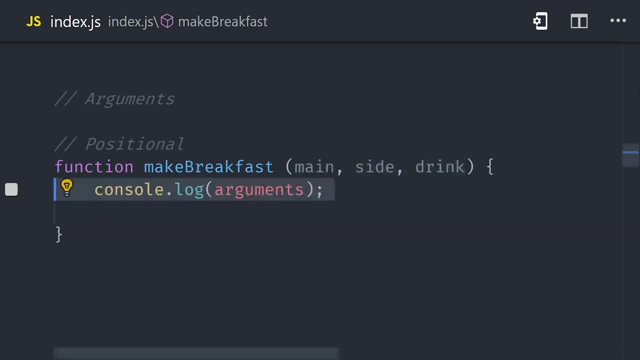 to log those out at runtime. we can do consolelog arguments, which is a keyword built into JavaScript. This particular function takes three positional arguments and that means when you call this function you need to pass in your arguments in the right order. That's pretty manageable. 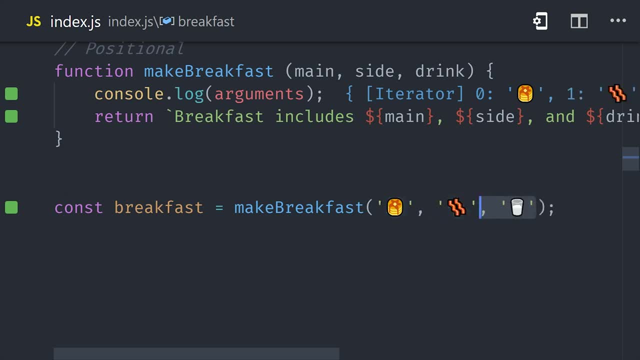 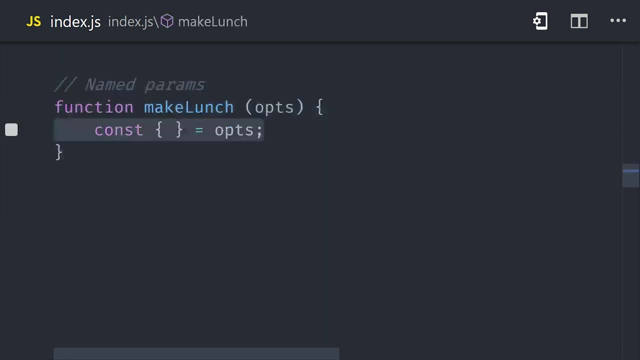 when you have three arguments, but imagine we had five or ten arguments to a function, Things would get out of hand very quickly. But when you run into a situation like that, a common solution is to use an object for named parameters, The makeLunch function. 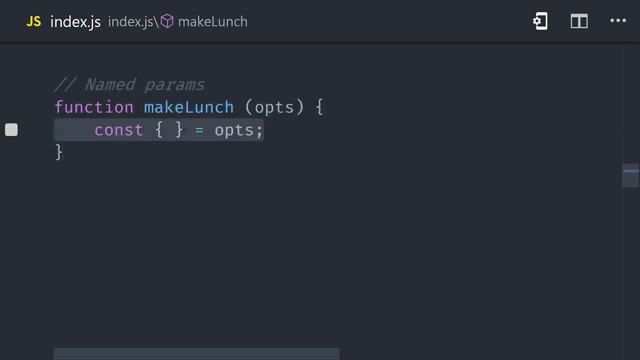 only has one single argument, but that argument is an object that can contain multiple values, And that means we can destructure the object or use it directly inside the function body. So with this approach, you don't have to worry about the function itself, you just need to. 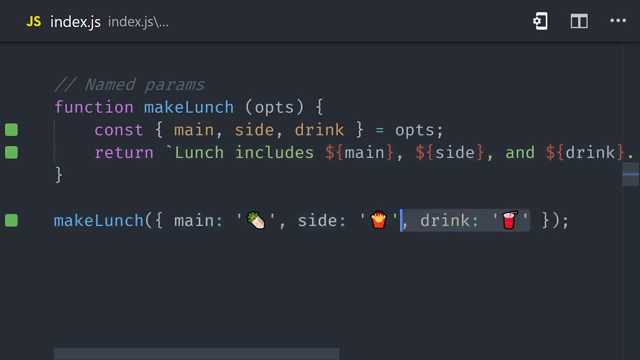 have to worry about the order of the arguments and also makes it more flexible to extend your code with non-breaking changes in the future. Now, one other trick that JavaScript has up its sleeve is rest parameters. In the makeDinner function, we have a single parameter, but it's preceded by three dots. That allows us. 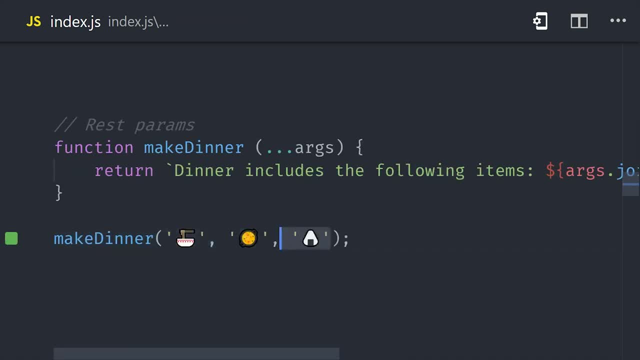 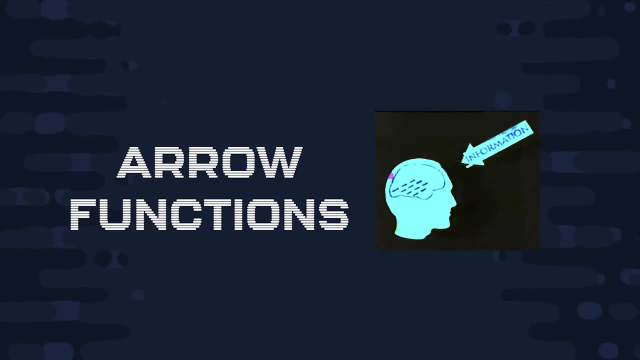 to call the function with multiple positioned arguments and then access them as an array inside the function body. Now, at this point, we've only been looking at the function keyword, but there's actually a more compact and concise way to write your functions, and that's using the arrow syntax. 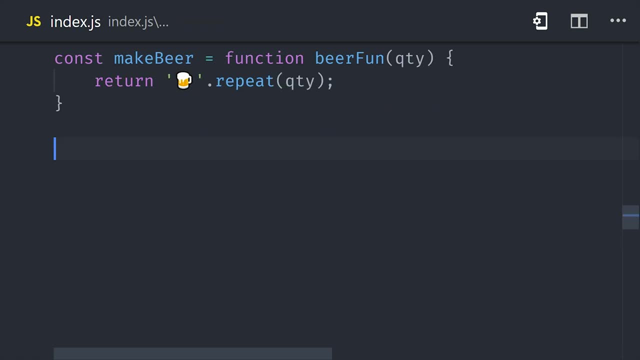 Let's go ahead and refactor one of our earlier function expressions to use the arrow syntax. We start with a variable to provide a name, then we have parentheses with the parameters to the function and then we have an arrow that points to the function body. 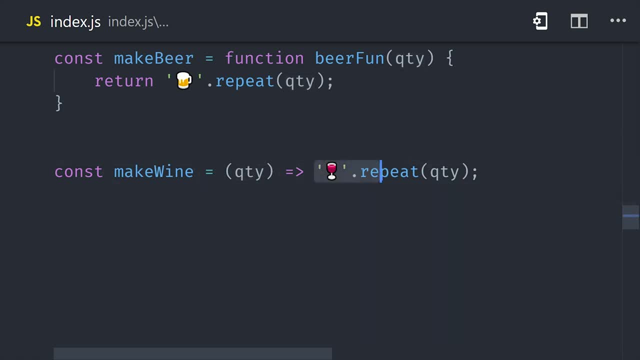 A cool thing about this syntax is that if you omit curly braces, then it will implicitly return that value from the function, and that means that three lines of code now become one. Now, if you have additional work to do inside the function, you can still add brackets. 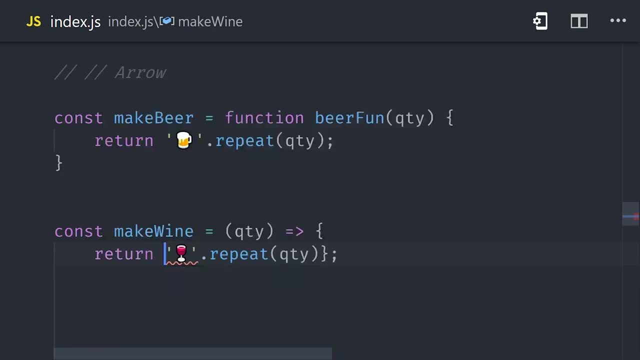 in which case you would still need to add a return statement to return a value from it. There are a couple of other characteristics that you should know. First of all, they will always be expressions, and that means you can't simply declare an arrow function in your code like this: 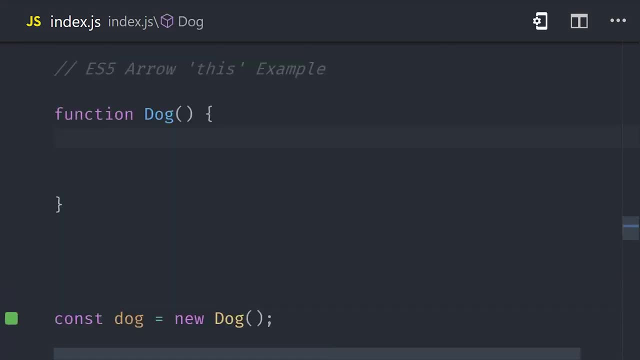 And the other big thing is that they don't have their own this object. Now, we're not going to get into this in this video, because there will be an entire video dedicated to object-oriented JavaScript that covers this in much more detail, But here's a little history that you should know for right now. 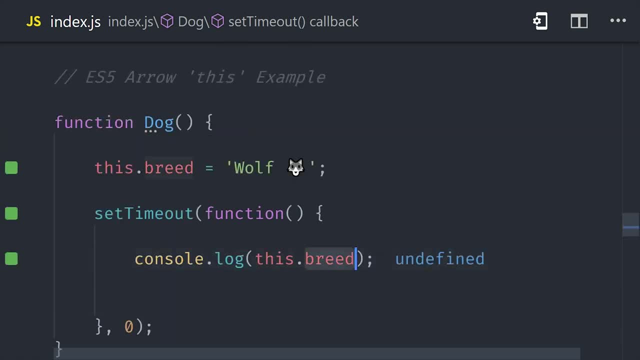 Prior to arrow functions, every new function would have its own this context that was based on how that function was called, And the reason this is important is because you might want to remember that every new function would have its own this context that was based on how that function was called. 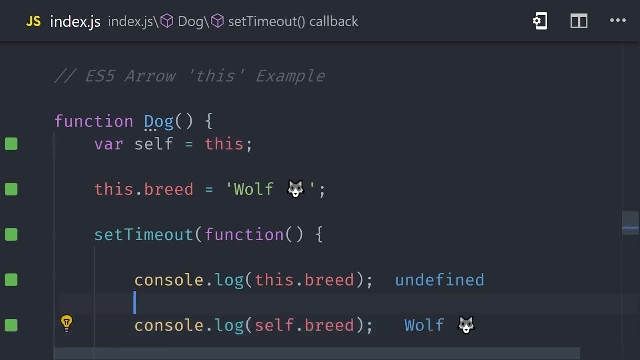 Because you might see older code where you have a function that defines a variable named self that is equal to this, And the reason you see code like this is because JavaScript will close over that variable and allow you to reference it consistently in other functions. For example, if we define a property on this function, we can now reference it using the. 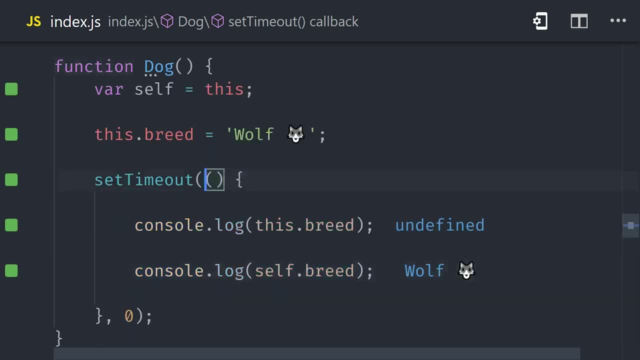 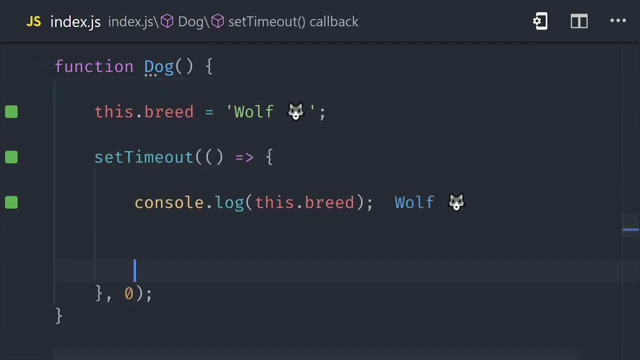 self variable in other functions. But the great thing about arrow functions is that we no longer need this ridiculousness. We can just use an arrow function, get rid of the self variable and we're good to go. Now that's more information than you need to get started working with arrow functions. 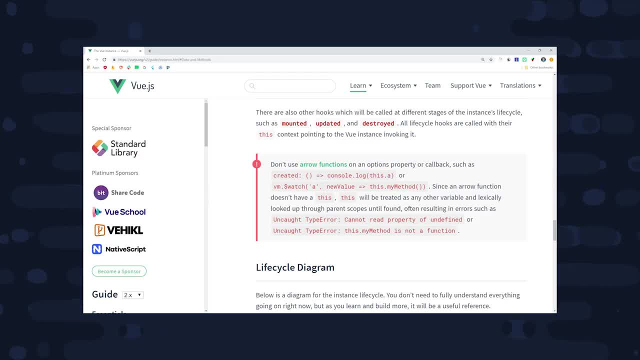 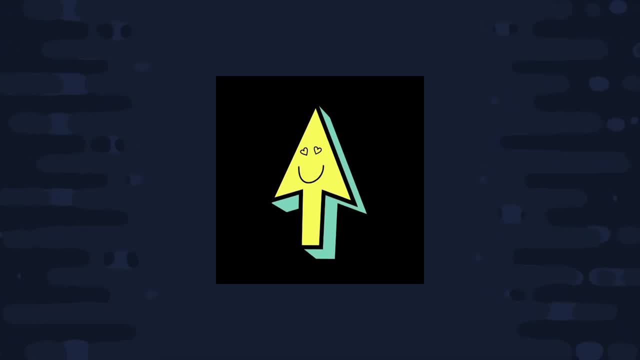 but it may come into play if you use a framework like Vue in particular. So always make sure to read the instruction manual that comes with your framework. And from here on out, we'll be mostly using arrow functions, because I think you should prefer that syntax when possible. 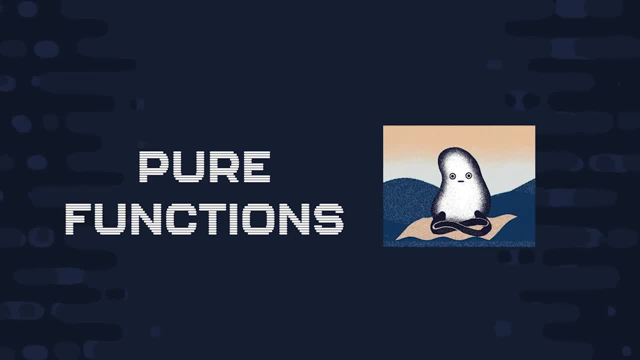 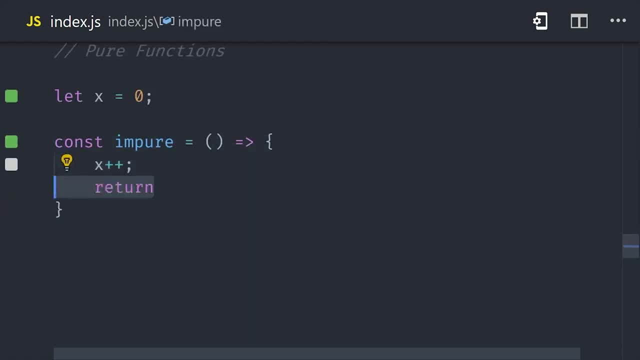 Now, another big thing you'll hear from thought leaders in the industry is the value of pure functions. But what is it that makes a function pure? Well, let's start by looking at an impure function. First we have a global variable, then we define our function, and that function mutates the 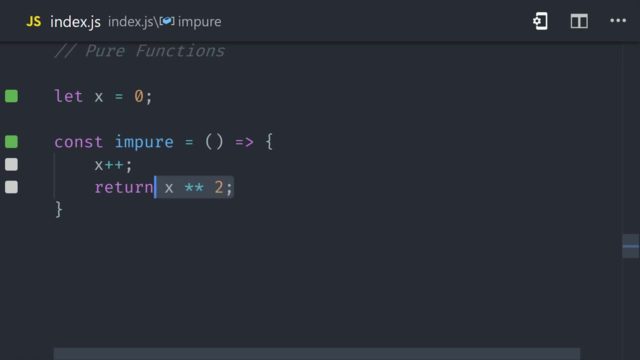 global variable and also uses it in its return value. What makes this code difficult to work with It's that it's operating on values outside of its local scope, And when you have functions that depend on and mutate global variables, it tends to create. 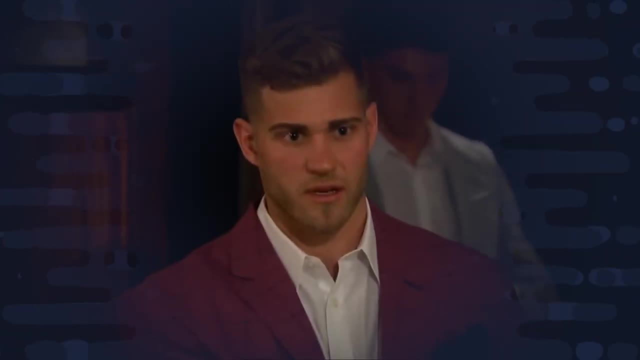 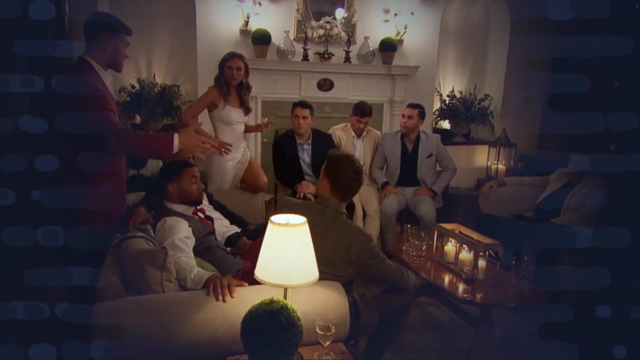 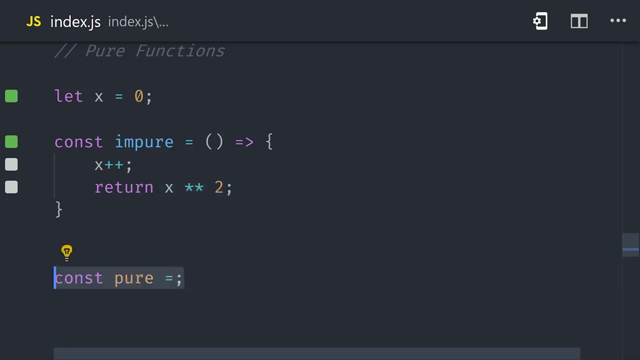 a lot of drama. So a pure function is one that only depends on its input parameters and only mutates variables within its local scope, And it should also not produce any side effects, And the end result is code that will always produce the same output given these same inputs. 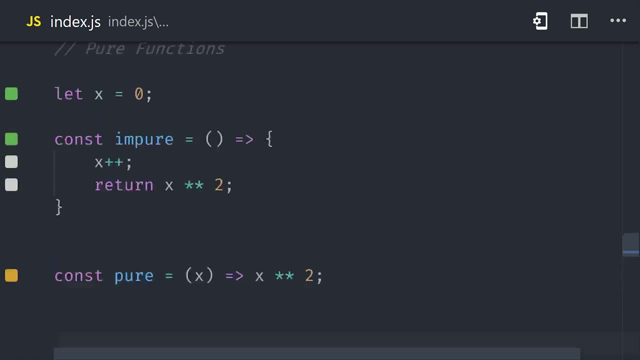 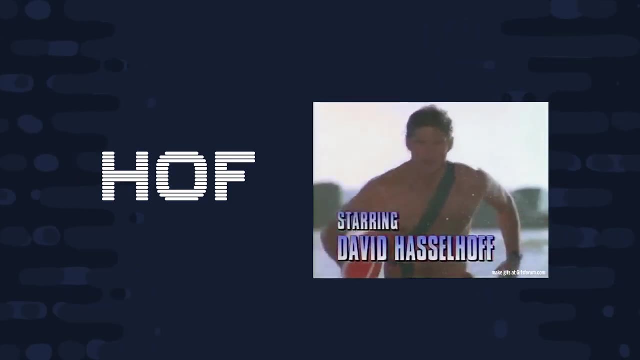 Code like that tends to be easier to test and also just easier to think about in general, Not to mention pure functions, will help you compose your applications as a collection of higher order functions. We learned in the very first video of this course that JavaScript supports first class. 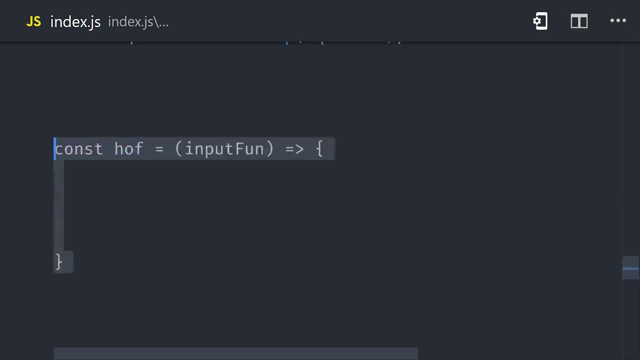 functions, And that means that you can pass functions as arguments to other functions or use functions as the return value from a function. So when you hear the term higher order function or higher order function, it means that you're using a function or higher order component in React. 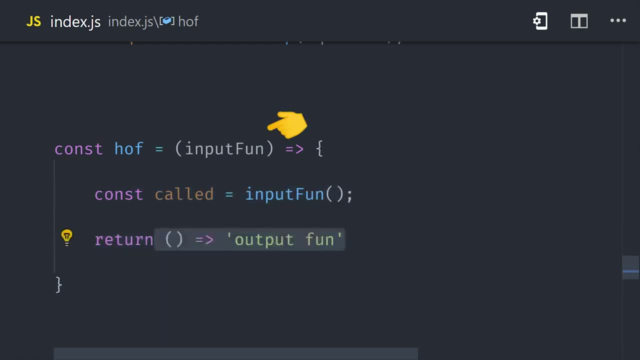 We're simply talking about functions that take other functions as their input arguments or return a new function when they're called. Using a function as an argument is a very common thing to do in JavaScript, especially when you start working with async code. We're not going to cover async stuff in this video, like promises and callbacks, because 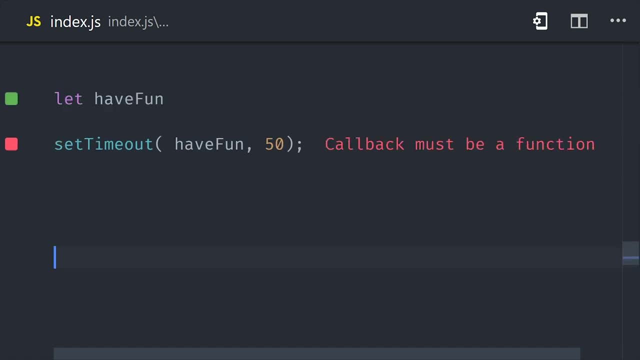 that deserves an entire video on its own, But a simple example of a higher order function is the setTimeout function that's built into JavaScript. It allows you to execute code after a specific delay, and it achieves this by taking a function as its first argument and then the number of seconds that you want to delay as the second. 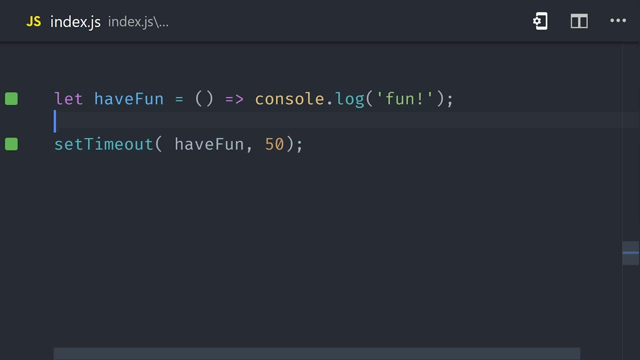 argument. We don't want to immediately execute the function that we pass to the setTimeout. Instead, we wait for the delay and then the JavaScript engine will call that function later, Hence the name callback function, And you'll see code like this all over the place in modern JavaScript. 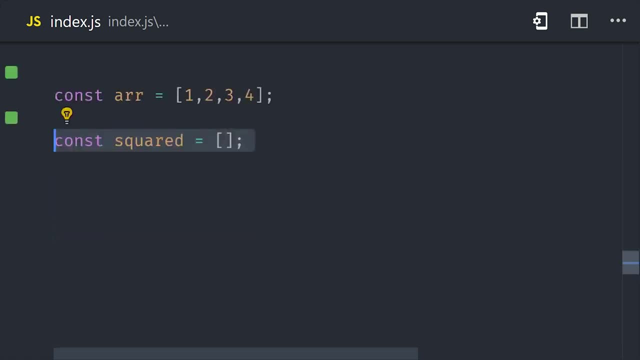 Another thing we can do with functional code is replace traditional for loops. As you can see in this example, we are looping over an array and then we're mutating each item in that array with a new value. But in modern JavaScript we can achieve the same thing in a single line with array map. 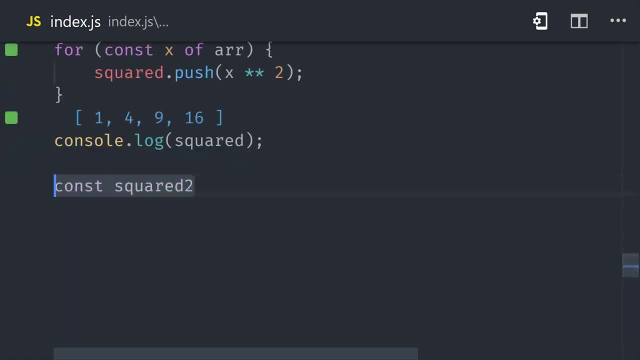 Which takes a function with a specific signature as its argument, And it will call this function for each item in the array. So x represents an individual item in the array, and then the return value from the function is what we want to transform it to. 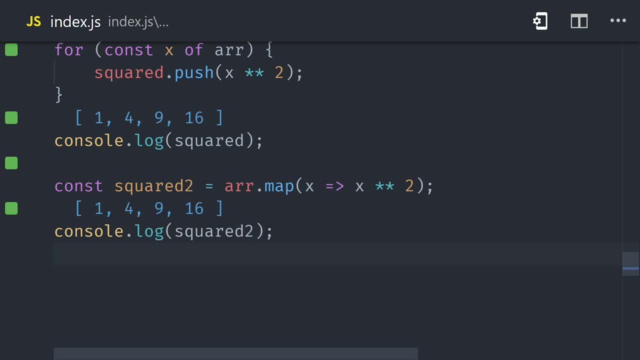 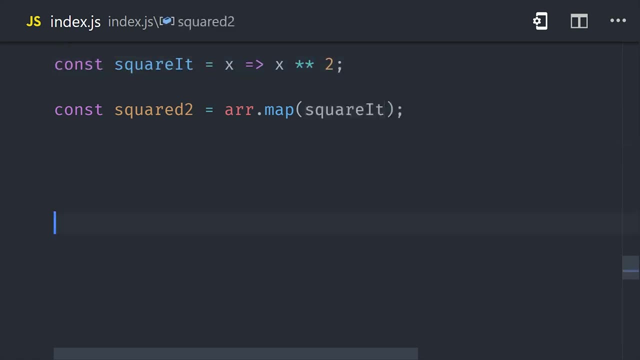 And this is especially awesome when combined with arrow functions, because you can achieve a lot with a single line of code, And if you want to reuse this code, you can simply set up a function expression with a descriptive name and then pass it as the argument to map. 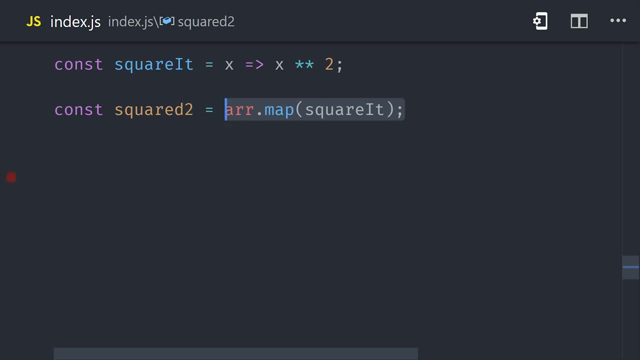 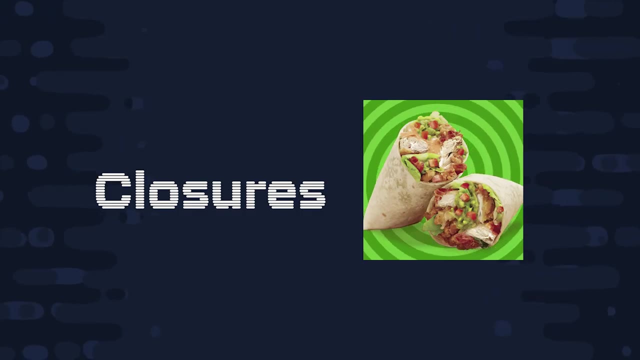 Now I should point out that these functional techniques tend to be less performant than a regular for loop, So I feel obligated to do that, Even though it's not going to matter in the majority of use cases. Now, another type of higher order function is one that returns a function. 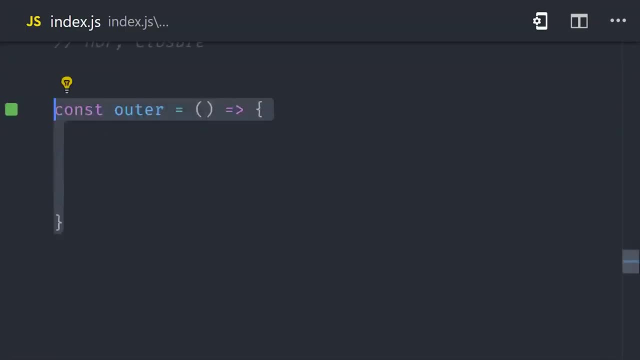 Now the thing you should know at this point is that whenever you define a function, you're also creating a lexical environment, And that sounds like a pretty scary term, but basically anything inside of curly braces is its own lexical environment. Now the inner function has a lexical environment that contains its own local variables, and 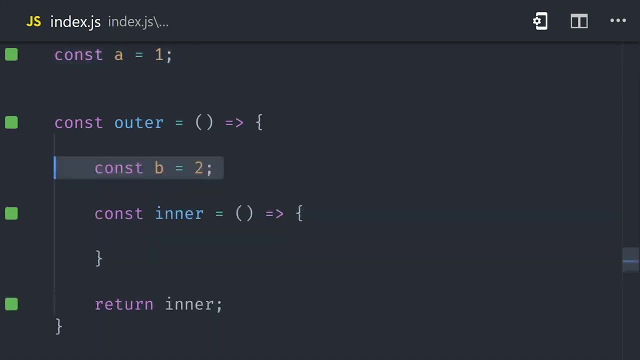 also a reference to the outer environment, which includes the outer function as well as the global script as well. Basically, what this boils down to is that the inner function can remember the local variables in the outer function, but the outer function can't look inward at the local variables. 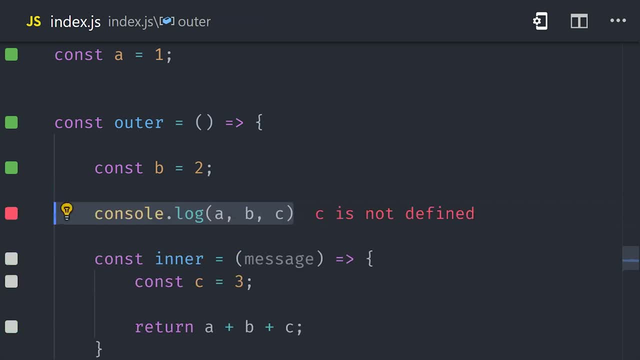 in the inner function, as we can see here from the undefined error Meow. let's go ahead and define a function called useCat that is a closure loosely inspired by React hooks. The outer function is its own lexical environment and will define local variables within it. 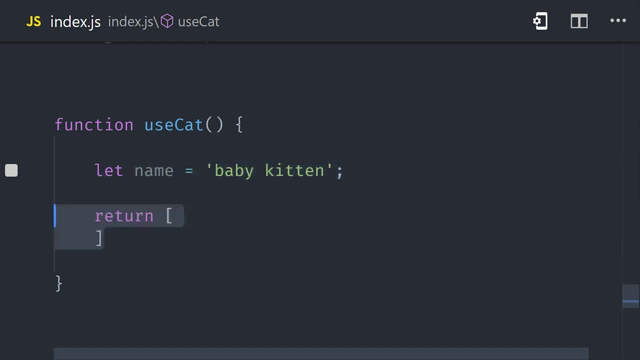 such as a default name when this function is first called, Then we'll return an array that itself contains two different functions. The first one just gets the name and prefixes it with meow Well, the second function is a setter that takes a new name as an argument and then sets 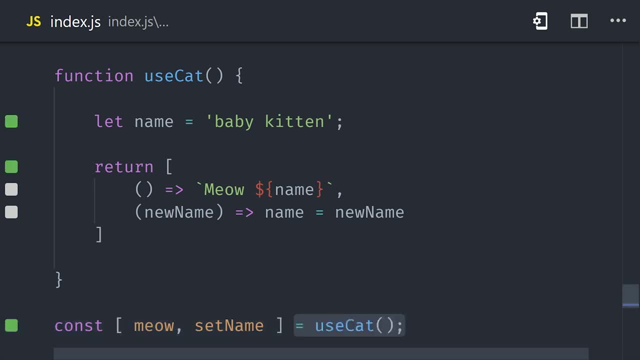 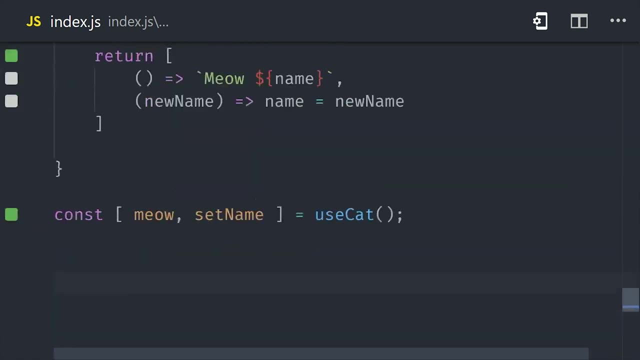 it as the name in the outer function And now we can use it in a way that resembles useState from React hooks. But the most important takeaway here is that the inner lexical environment or the inner functions in the array have access to the local variables in the outer useCat function. 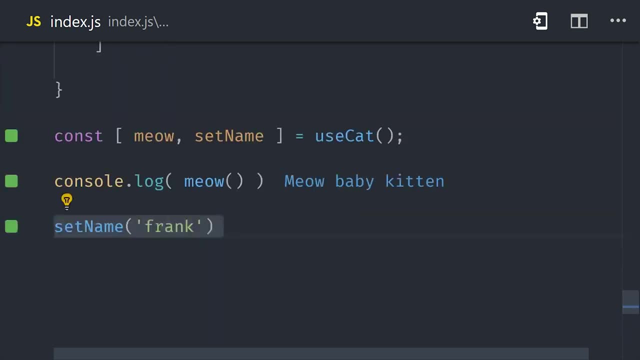 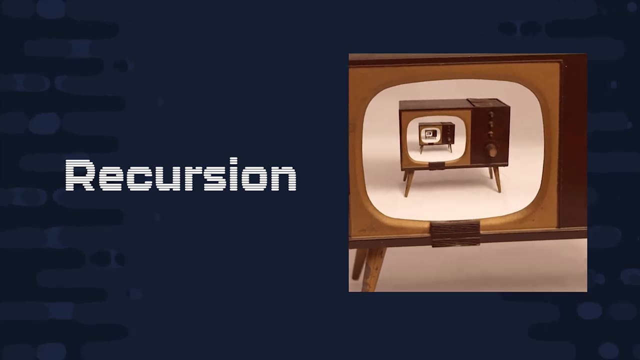 So I highly recommend that you practice this and get comfortable with closures, because you'll find them on both interview questions and in the real world. And speaking of interview questions, another thing you might encounter is recursion. In JavaScript, We call a function by simply defining a function and then calling it by name in the function. 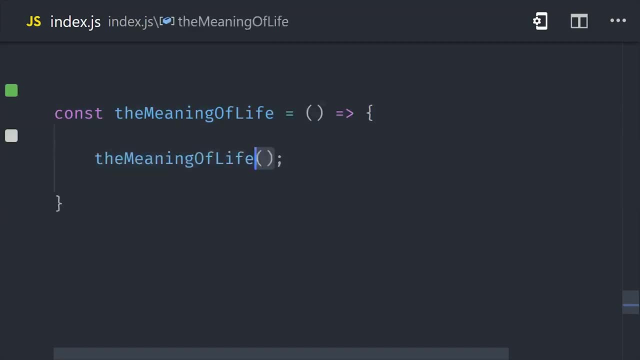 body. When this function encounters the function call, it's simply going to push another instance of this function on the call stack And in our case we have no stopping condition, which means it will do this forever in an infinite loop until we reach stack overflow.